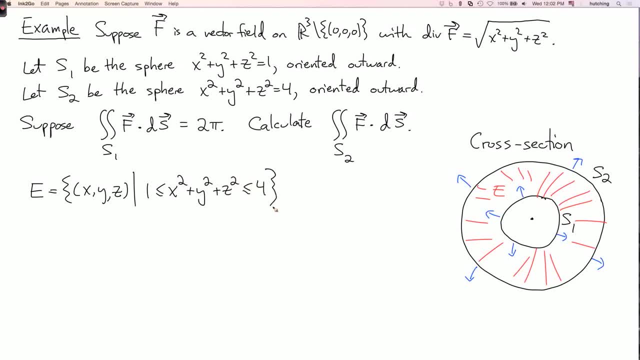 is less than or equal to 4.. And let's apply the divergence theorem to this solid region, e. So what does the divergence theorem say? It says that the triple integral over e of the divergence of f with respect to volume is equal to. and now the other side is, I have the flux over the boundary of e. 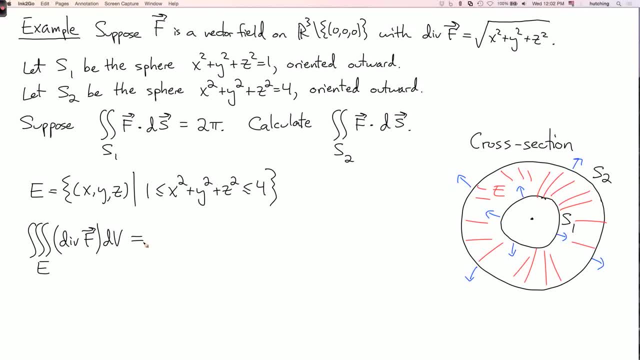 The boundary of e consists of the two surfaces s2 and s1. So on s2, I have the integral over s2 of f dot ds, And the other surface is s1. And I'm going to have minus the double integral over s1 of f dot ds. 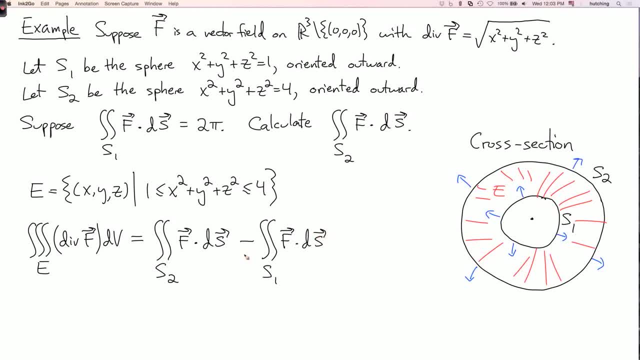 Now why did I put a minus sign here? So this is the part you have to be really careful about, namely the orientations of the surfaces. So in the divergence theorem you have to orient the surfaces, pointing out of the of the solid region E. okay, 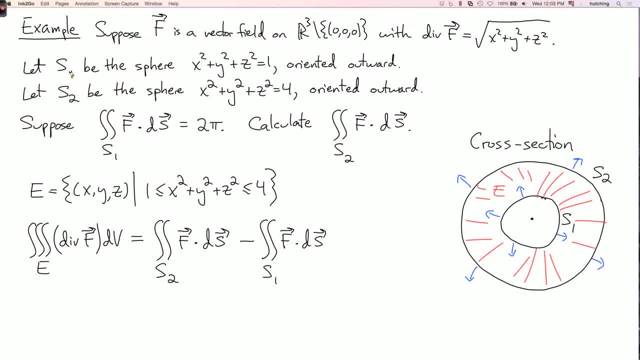 Now we're given orientations of S1 and S2, which we fixed at the beginning. So this is S2, oriented out, I'll say out from the origin, And this is S1, which is oriented out from the origin, But in the divergence theorem. 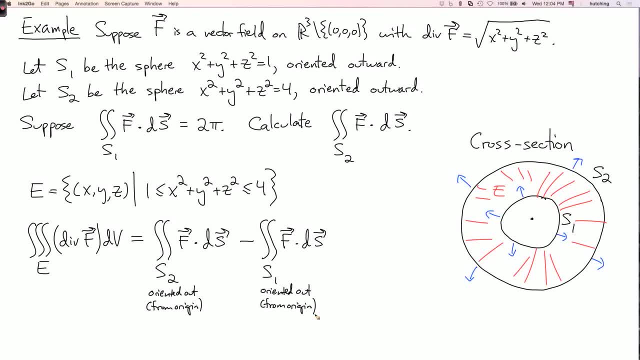 the surfaces are supposed to be oriented out of the solid region E. Now if you look at S2, there's no difference here, because S2 is oriented going outward from E, But S1, the given orientation, which is pointing away from the origin. 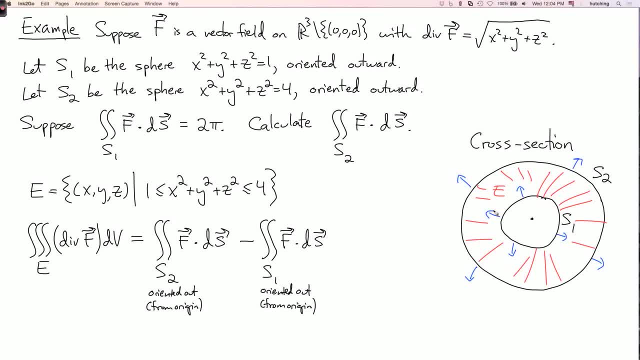 points in to the region E. So the orientation of S1 that we're given is the wrong orientation to use in the divergence theorem. So if you integrate with that orientation you'll get the wrong sign. So you just have to multiply by minus one to get it right. 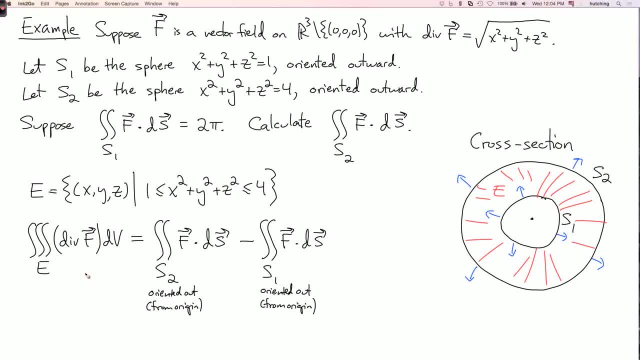 Okay, so this is what the divergence theorem tells us. Okay, and then? why is this useful? Well, this integral of S2 is what we're trying to find. So we want this And we're given. the flux over S1 is equal to two pi. 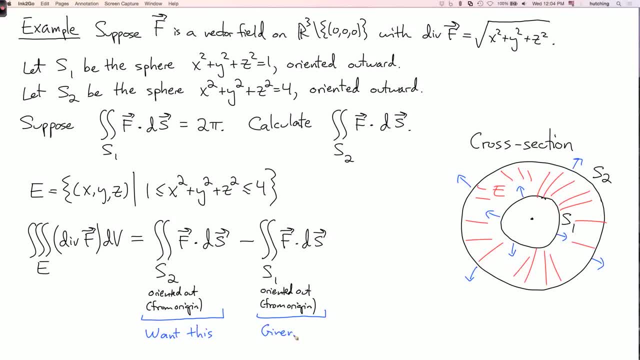 So we're given that this is equal to two pi. And then, to complete the problem, I just need to do this divergence integral. So we need to calculate this, Okay, and then the answer will be two pi plus this divergence integral. So that's just one pi plus two pi times two pi. 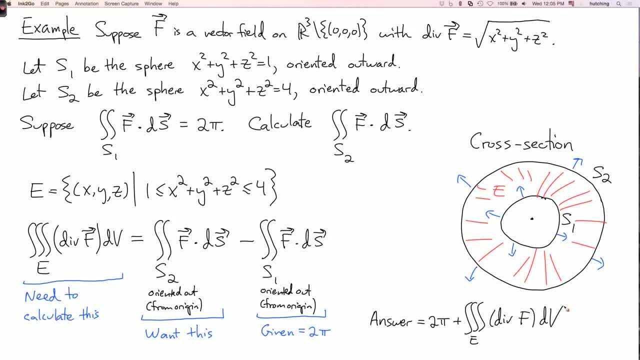 And then let's say: okay, so what is the derivative of S1?? It's just one pi plus two pi. Alright, so we just have to calculate this integral. So we're just going to need to compute this integral as the integral for S1.. 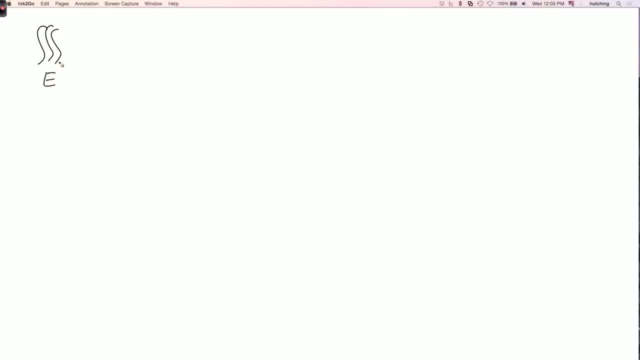 Because it's like we're going to have to do it with a tangent after tangent, So we're going to have to find the integral to be equal to the product of S1, or the product of S2, or the product of S3,. 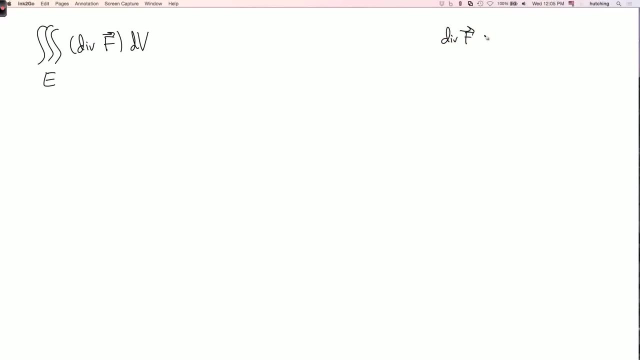 that the divergence of f is the square root of x squared plus y squared plus z squared, and the region E is defined by the inequality: 1 is less than or equal to x squared plus y squared plus z squared is less than or equal to 4.. 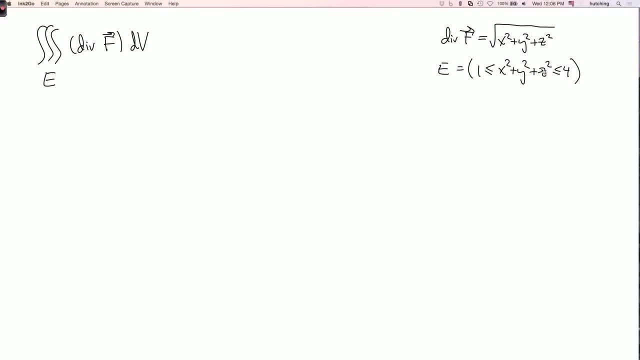 Now, since we have all these x squared plus y squared plus z squareds here, that suggests that we should try using spherical coordinates. So in spherical coordinates, the divergence of f is simply rho, the distance to the origin, and E is given by. 1, is less than or equal to rho is less than or equal to 2, while theta. 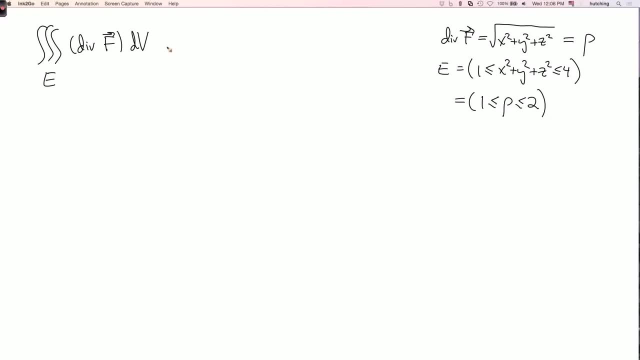 and phi can be anything. So in spherical coordinates this is the integral, as phi goes from 0 to pi, theta goes from 0 to 2 pi and rho goes from 1 to 2, and the divergence is rho. and then we have the magnification. 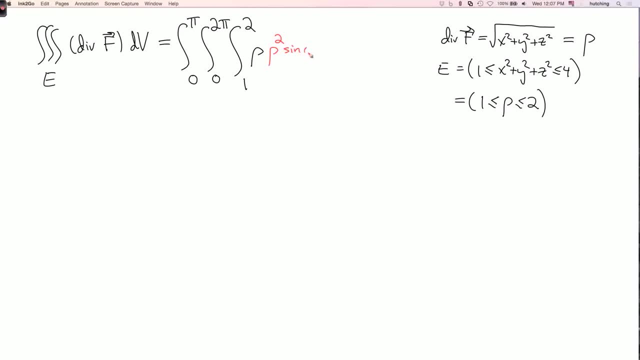 factor: rho squared sine phi, and then we have d rho d theta d phi. Okay, so when I do the rho integral, I have to integrate rho cubed sine phi. the sine phi is like a constant, so I get rho to the fourth over 4 sine phi evaluated at rho equals 2 and rho equals 1, d theta d phi. 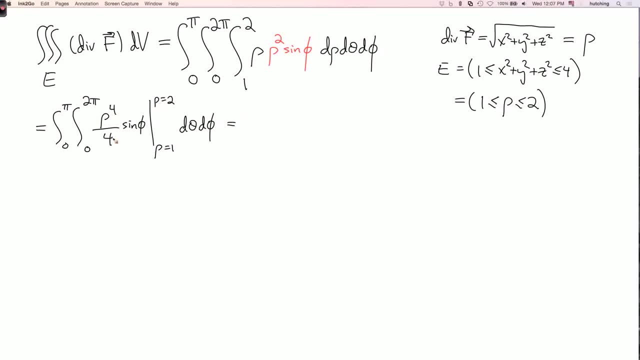 So this is: if I take rho to the fourth over 4, at 2 and 1, I'm going to get 16 over 4 minus 1 over 4, which is 15 over 4.. So let's just pull that out here. 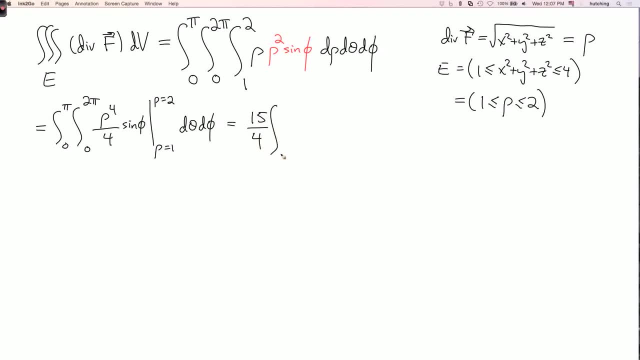 So I get 15 over 4 integral from 0 to pi. integral from 0 to 2 pi of sine phi d theta d phi. and when I do the theta integral I just multiply by 2 pi. So I get 15 pi over 2 integral from 0 to pi sine phi d phi. 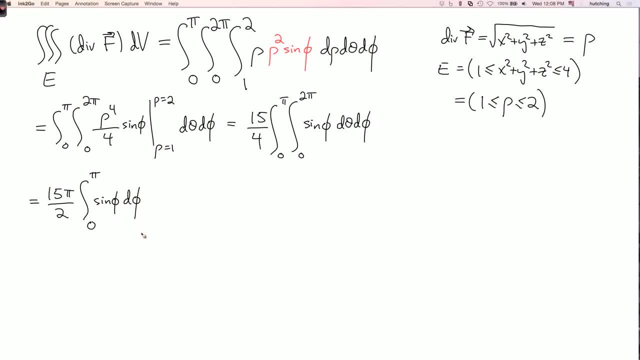 And if you've been doing these kinds of integrals through this whole course, you can probably immediately tell me that the integral of sine phi from 0 to pi is 2, so we get 15 pi. So that is this triple integral, and then remember. 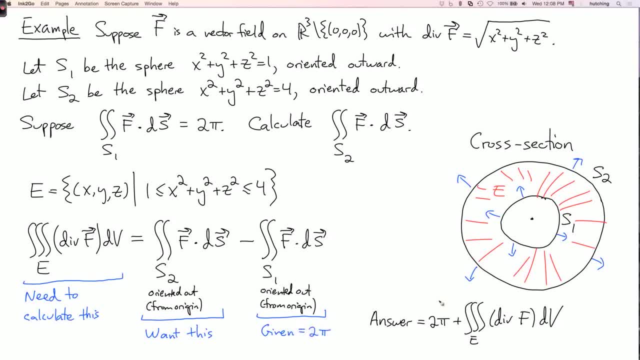 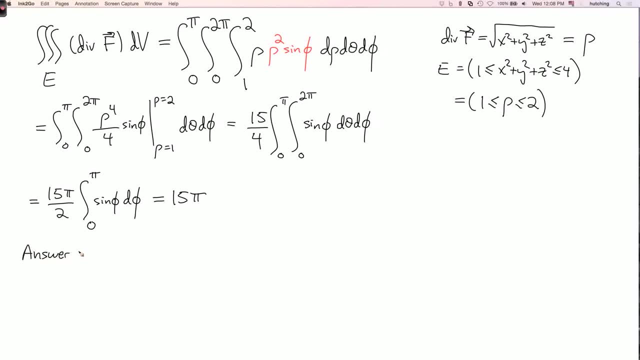 to get the answer, I needed to take that integral and add 2 pi to it. So the answer is 2 pi plus 15 pi, which is 17 pi. Okay, so that's nice. Now a word of warning here. 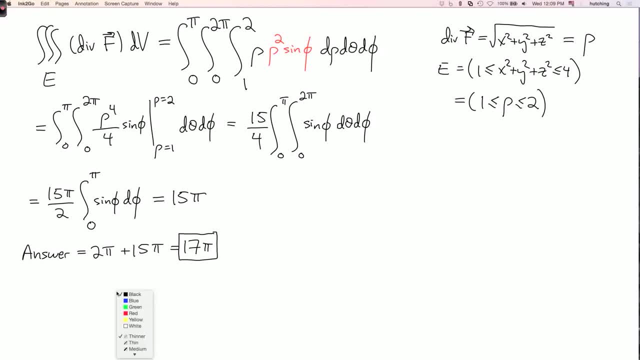 Let me show you the wrong way to do this problem, which will give you the wrong answer. So the wrong approach Is to apply the divergence theorem to the ball of radius 2.. So the ball x squared plus y squared plus z squared is less than or equal to 4.. 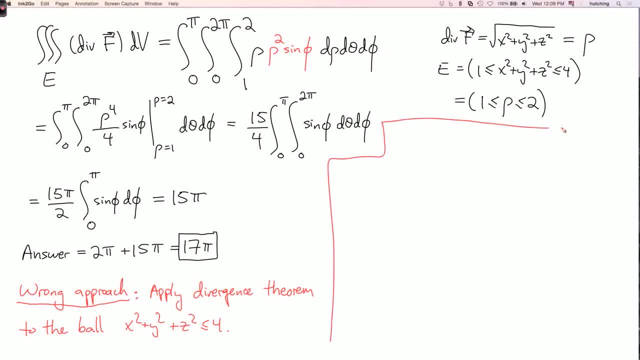 So if you try to do it this way, well, here's the ball in cross-section and its boundary is the surface S2, oriented outward. So if you apply the divergence theorem here, I'll keep writing in red to indicate that this is wrong. 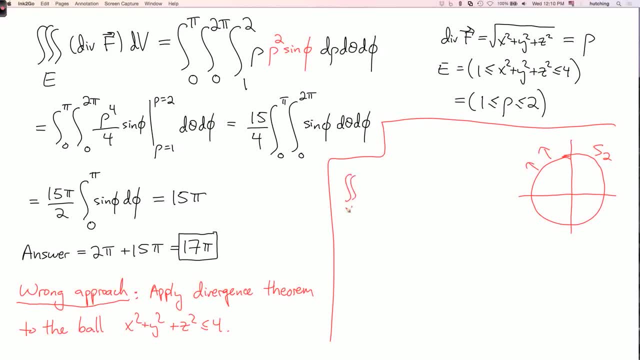 So you would get that the double integral over S2 of f, dot ds is a triple integral over this whole ball. Let's call it b. There's a triple integral over this ball of div, f dv. Now this ball is similar to the region we integrated over before. 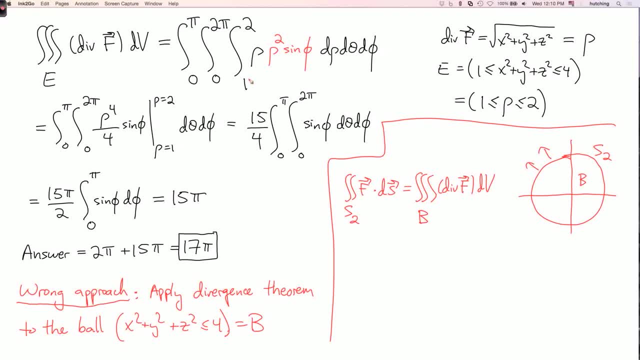 The only difference is that now rho goes from 0 to 2 instead of from 1 to 2.. So b is also where rho is less than or equal to 2.. So if you do it this way, when you do the rho integral, 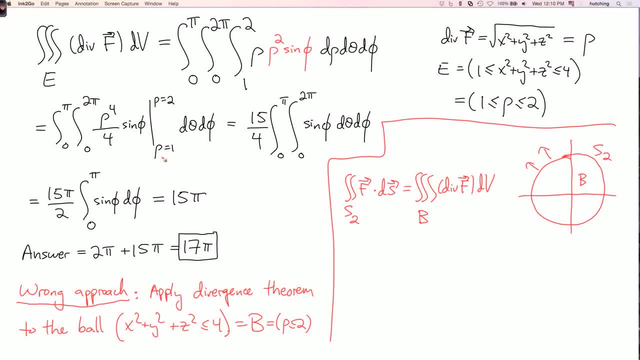 instead of evaluating at rho equals 1, here, you'll evaluate at rho equals 0.. And this 15 over 4 will turn into a 16 over 4.. So you'll just replace the 15 with a 16. So you'll get 16 pi. 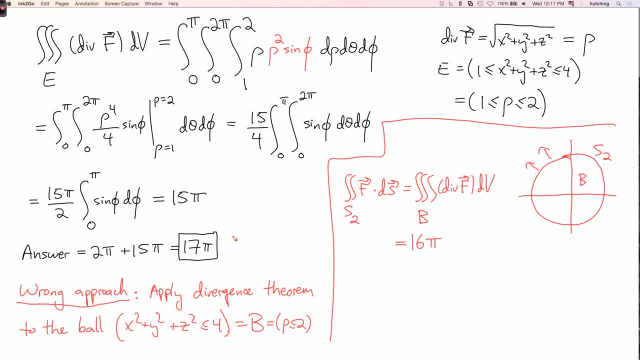 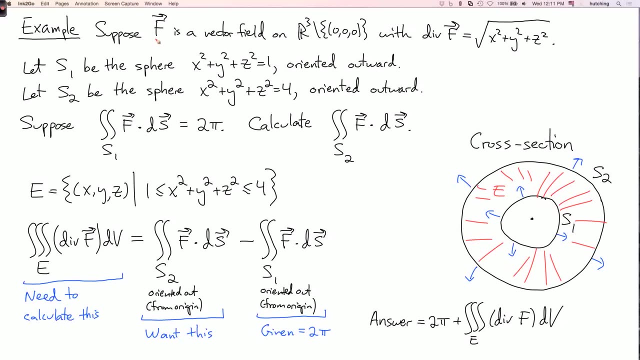 And that's wrong, because the answer is 17 pi. So what's going on here? Why is the divergence theorem giving us the wrong answer now? Well, let's look carefully here. So f is a vector field, And where is this vector field defined? 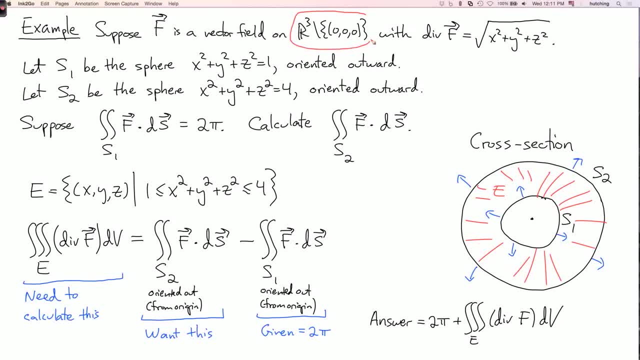 It's defined on r3 minus the origin. Now, if you're going to apply the divergence theorem, the vector field needs to be defined on the entire solid region E that you're using. Now. when we did the problem the first time, that was okay, because we took E to be the region. 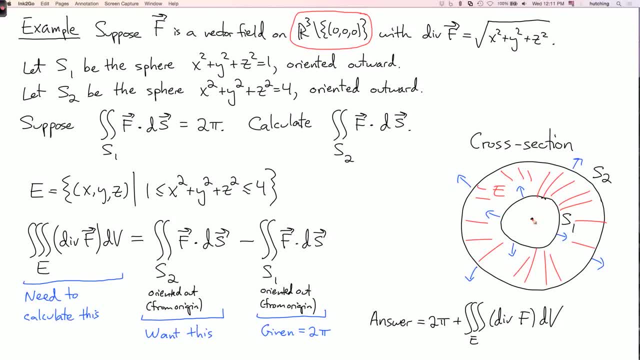 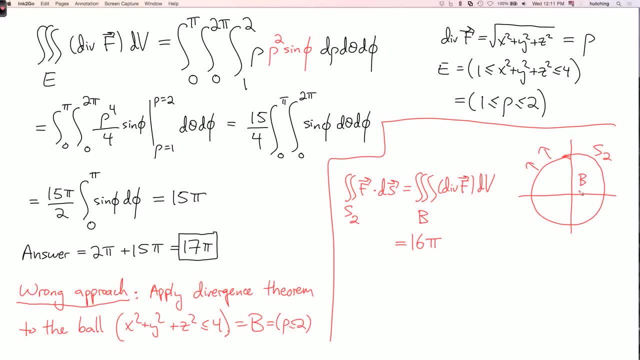 where rho goes from 1 to 2. That does not include the origin. so there's no problem there. But my second attempt: I used a ball, which includes the origin, where the vector field is not defined. So this is not valid because the vector field f is not defined.